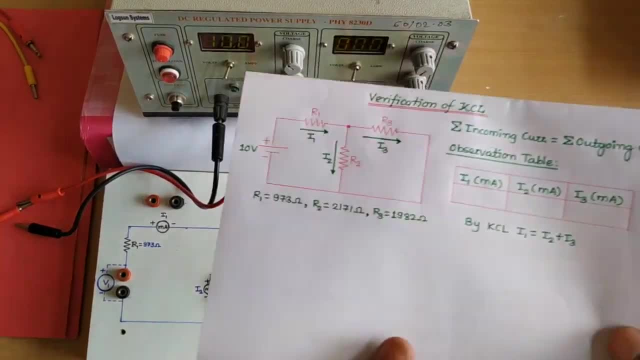 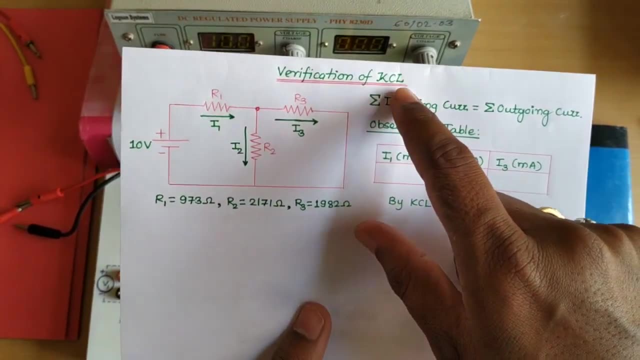 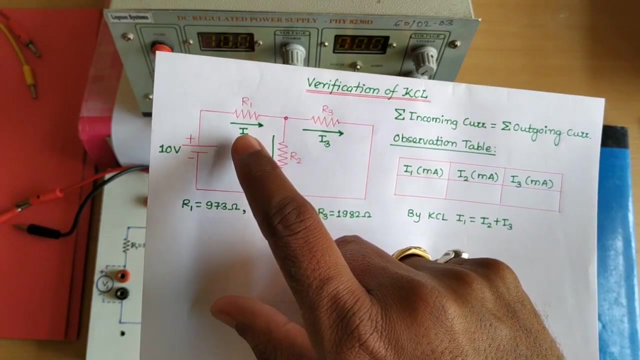 Hello friends and welcome back. Today we are performing experiment on KCL. KCL stands for Kirchhoff's current law. So in this experiment we will verify the KCL by using this T type network. So here you can find we are having three resistances: R1, R2 and R3 and current. 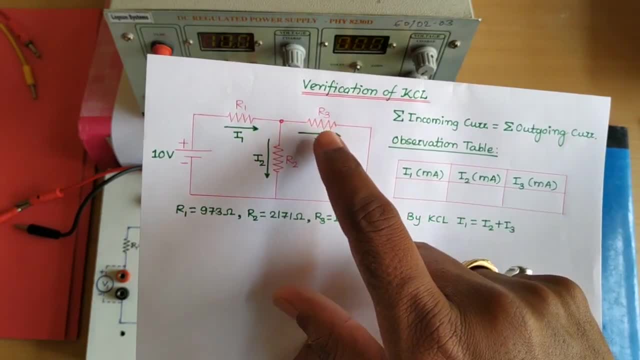 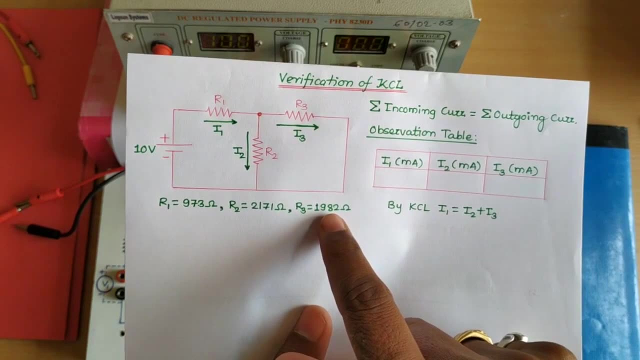 flowing through them. we are calling as I1, I2 and I3 respectively, And from this side we are applying 10 volt. Okay, so this is your supply voltage And these are the resistance values. we have already measured those resistance values by using ohm meter. Okay, KCL states. 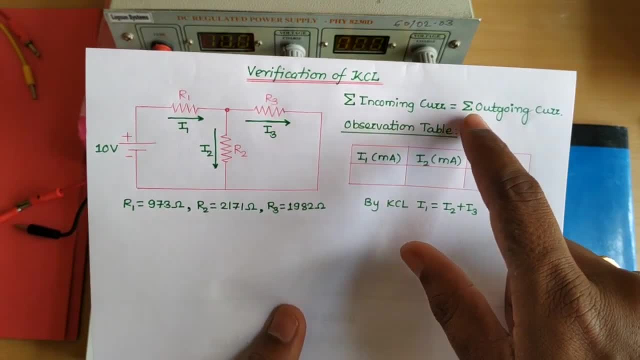 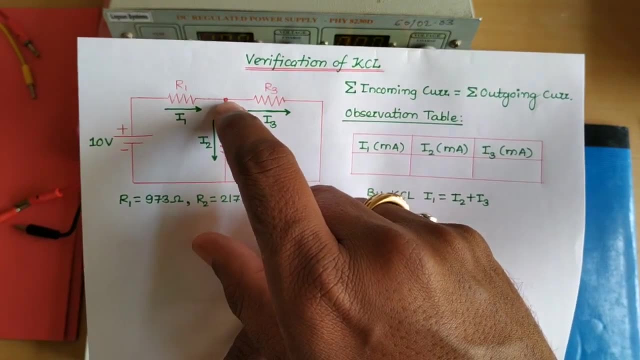 that algebraic sum of all incoming current is equal to algebraic sum of all outgoing currents at any node. So far as our circuit is concerned, we are having node Okay, so at this node we are applying KCL. So what are the incoming currents? I1 is incoming. 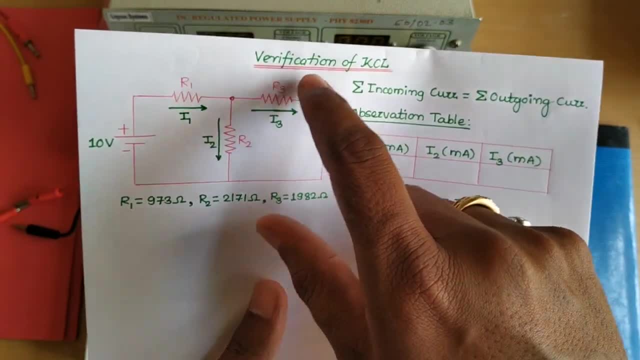 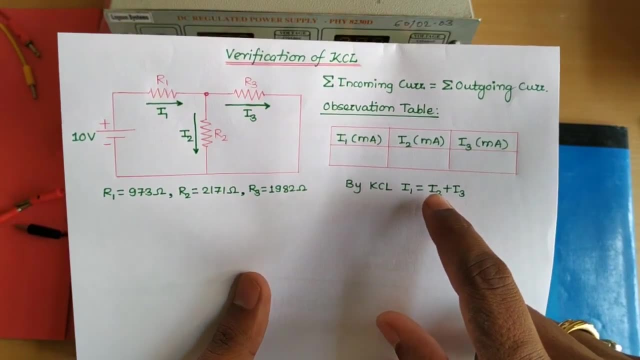 current and I2 and I3 are outgoing currents. So, as per the statement of KCL, what we are getting I1 means incoming current. So, as per the statement of KCL, what we are getting- I1 means incoming current- is equal to outgoing current, I2 plus I3.. Okay, so we have to measure. 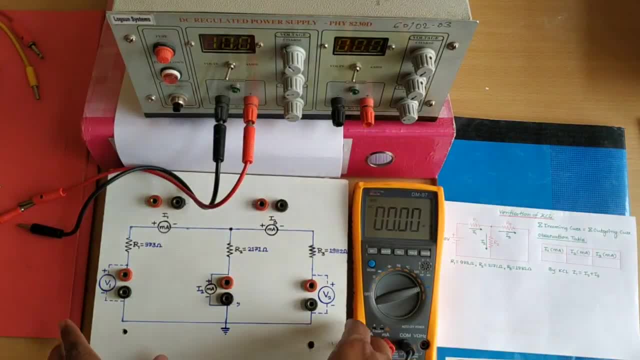 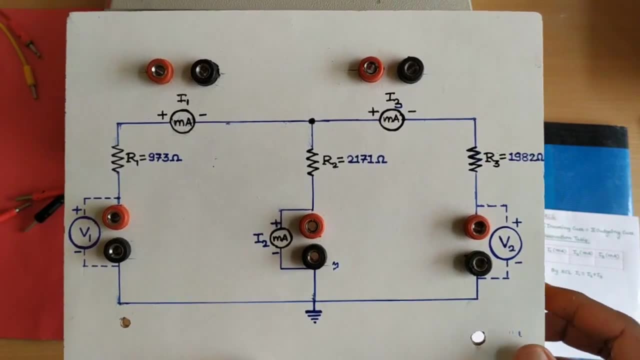 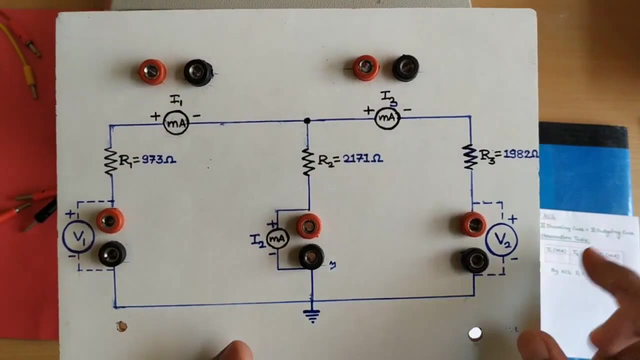 I1, I2 and I3.. So for this experiment we are using this experimental setup. Okay so you are already acquainted with this experimental setup. I have performed a number of experiments by using this experimental board. The links are available in the description. Okay so. 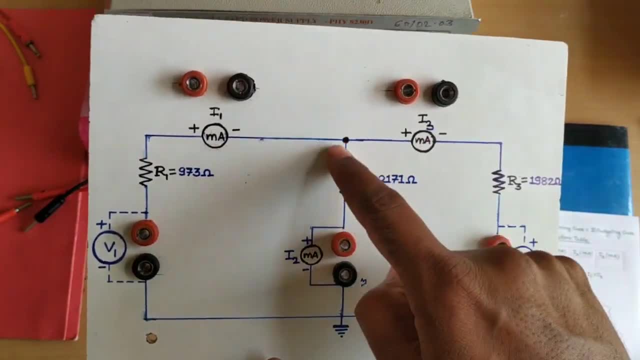 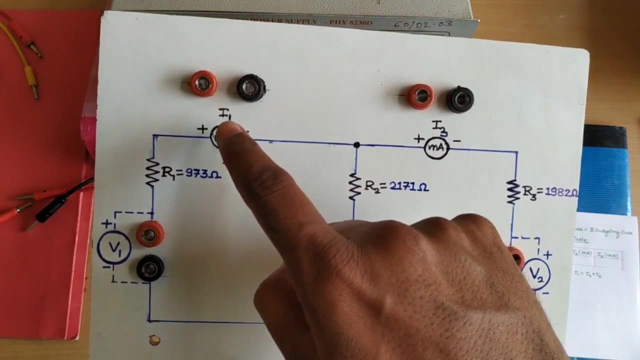 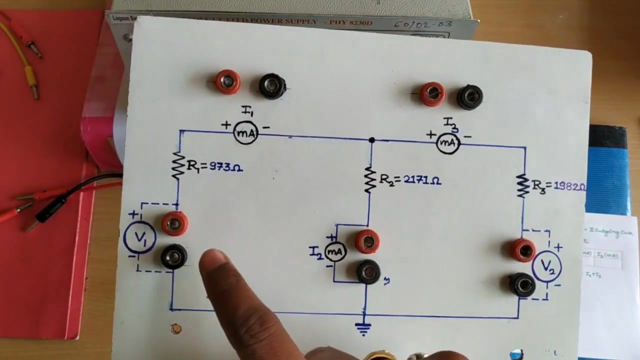 here you can find that we are having this T type network. Okay, R1, R2 and R3 we are using In order to measure current flowing through these resistors. we are using I1, I2 and I3.. So these are the connectors where we are externally connecting emitters And in this we are having 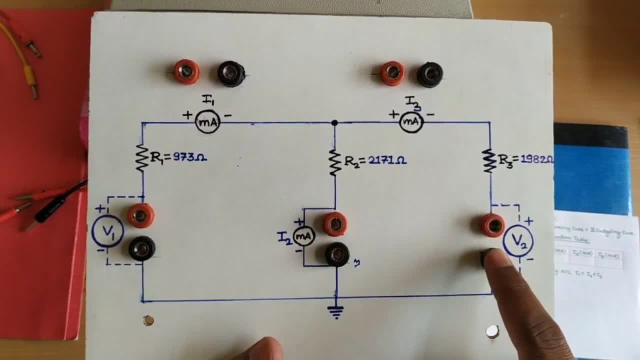 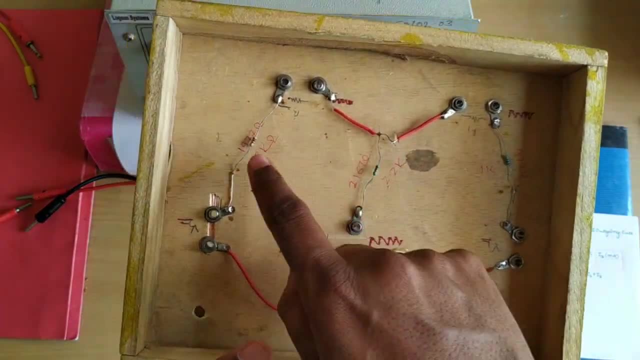 two loops, So at a time we can apply two voltages. Okay, but as per our circuit diagram, we need only one voltage source, And from the backside you can see that we have already soldered desired value of resistances. Okay, so this is about this experimental board. And now. 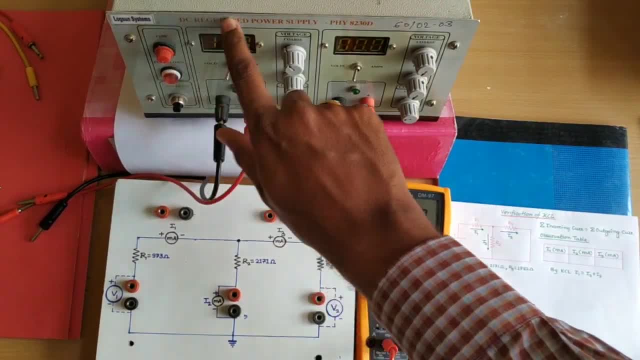 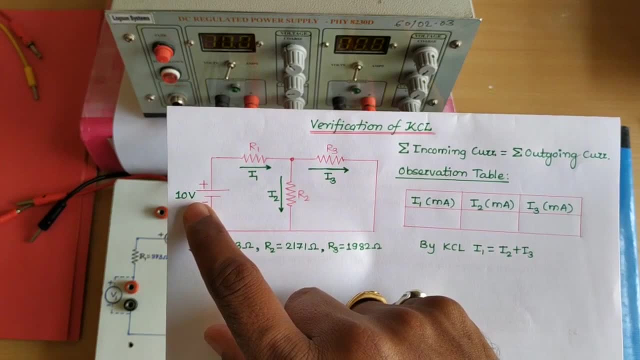 we have to provide power to this circuit. we are using this DC regulated power supply. Okay, so, as per our circuit diagram, what voltage we are using over here? 10V we are using as a supply voltage. so here you can see that I already set the voltage to 10V. 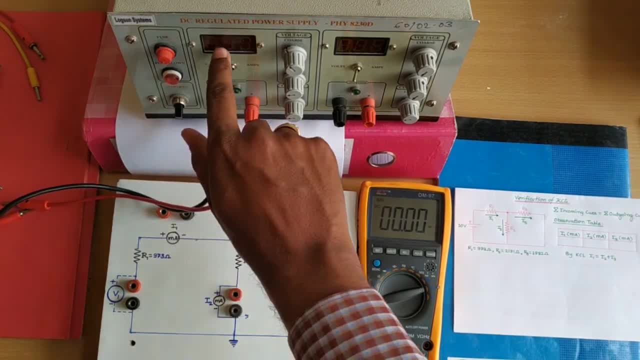 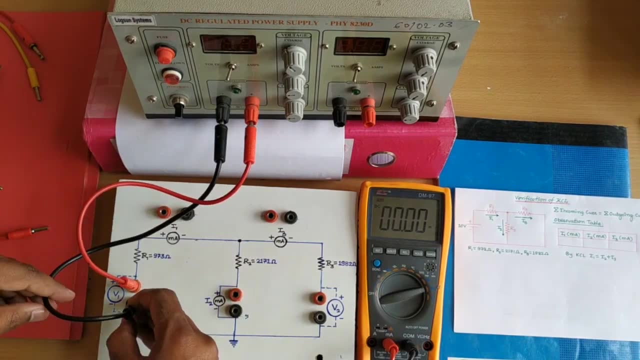 Let us start the connections. So first of all turn off the power supply. First you have to set the desired voltage and then connect the power supply in the circuit. So here I have connected the positive and negative, okay, the second supply we are not using, H5 is the current, direct current and the power supply is anijdKC and the壓 chaos violated. 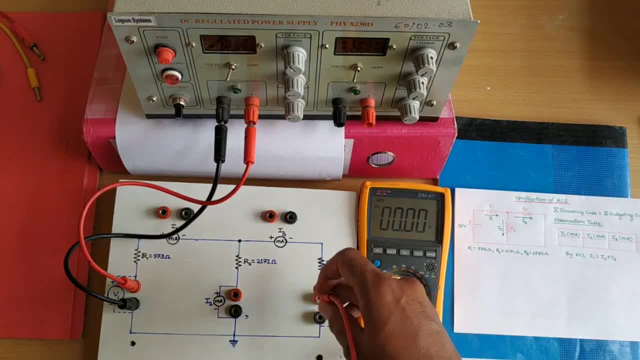 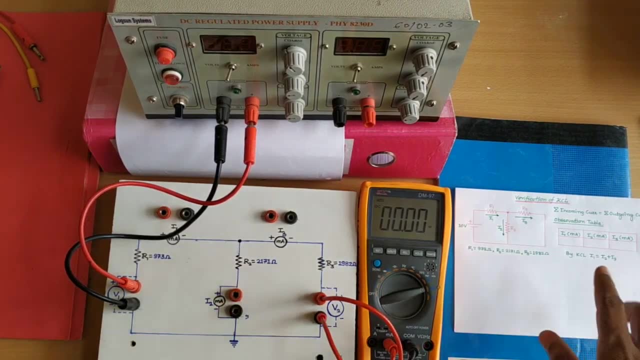 okay, so what i will do? i will short these two terminals. so these two terminals are shorted. it means what second voltage is not applied. okay, then we have to measure three currents, but we are having single emitter, so one by one we will measure the currents. so first of all, suppose 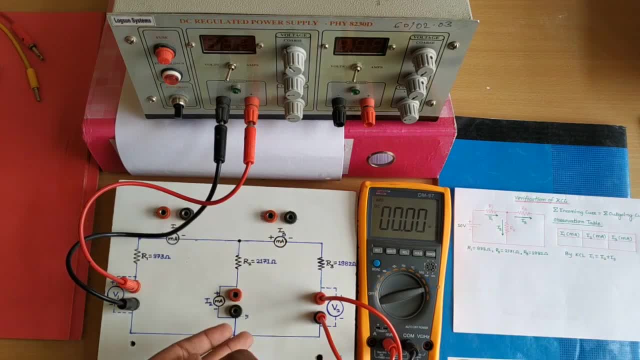 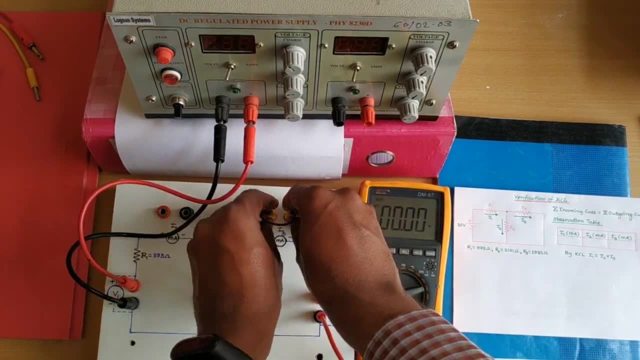 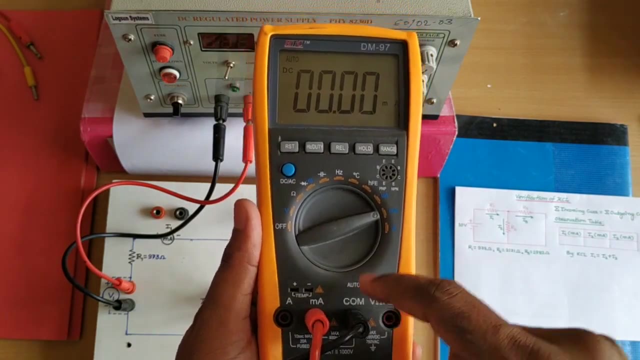 i am measuring i1, so i at that time i2 and i3 are not needed, so i will connect short circuit over here. okay, i have selected milliampere range over here. red probe is connected in milliampere, black probe is connected in common and here we have selected dc, so this emitter can be used for. 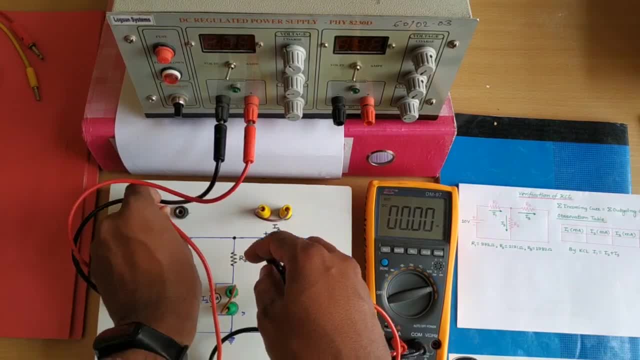 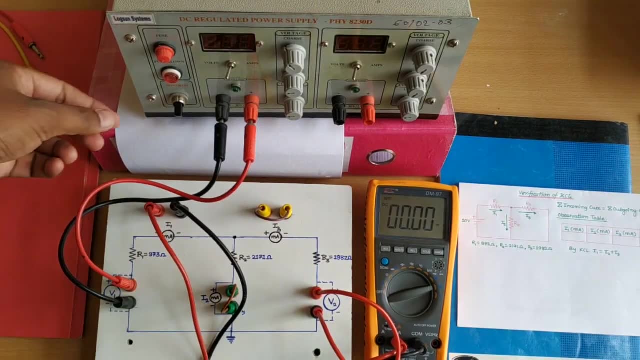 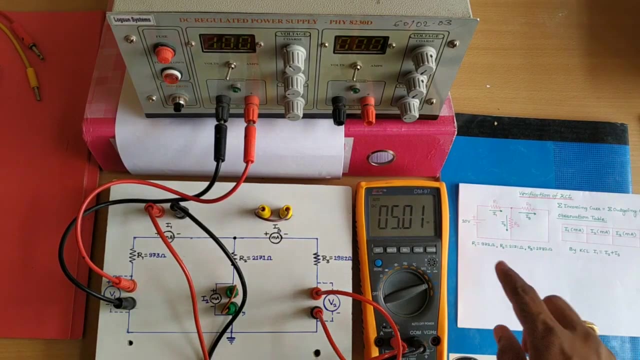 measurement of i1. so what i will do: positive, i will connect over here, and negative is connected over here. positive and negative. so here what we will get: i1. now your experimental setup is ready. just turn on the power supply and observe this reading: okay, okay. so as soon as i turn on the power supply, what value you are getting? 5.01 milliampere. so this is. 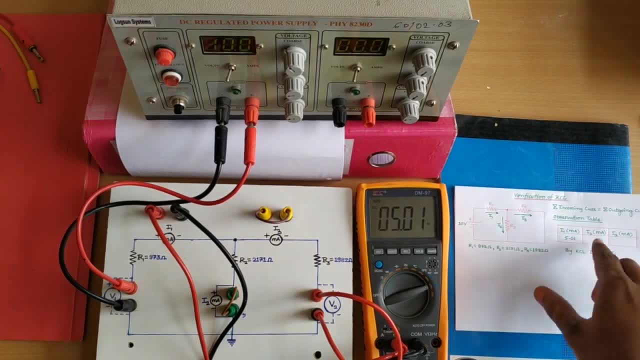 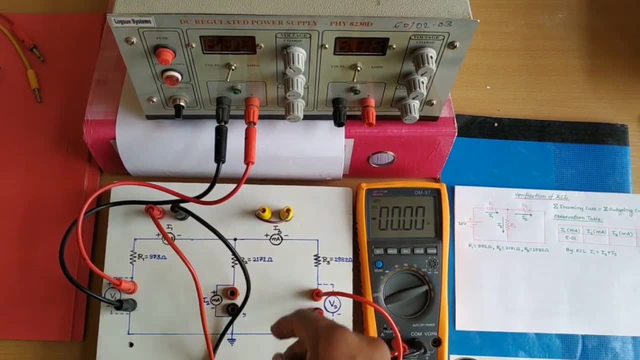 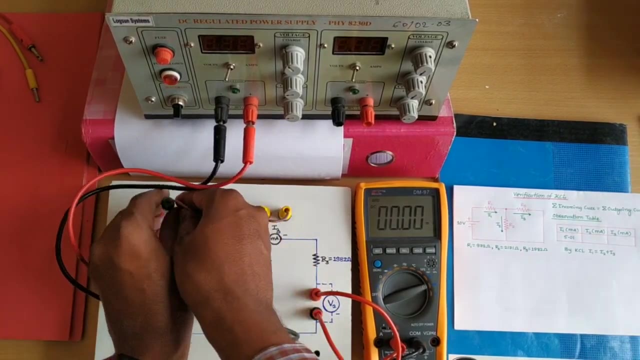 nothing but your i1. so we have noted i1. now we will note down i2. so what i will do? i will turn off the power supply. i will remove this open circuit- sorry, short circuit. i will connect the emitter over here so that i will get i2. now this is replaced by short circuit. okay, and again. 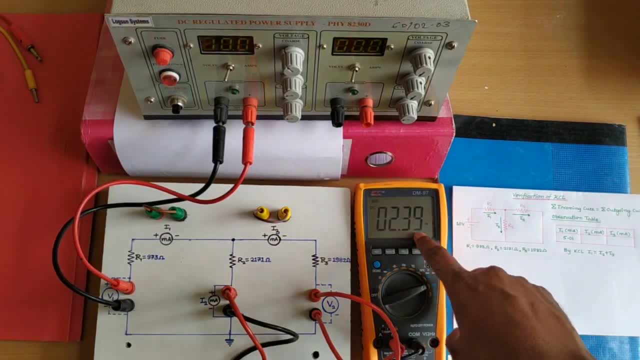 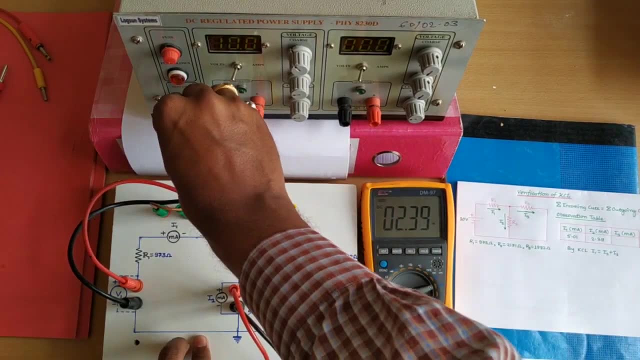 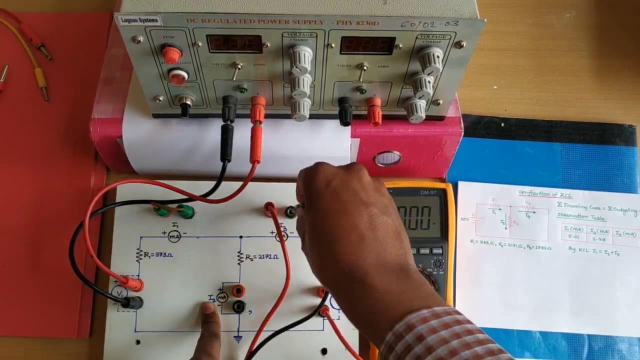 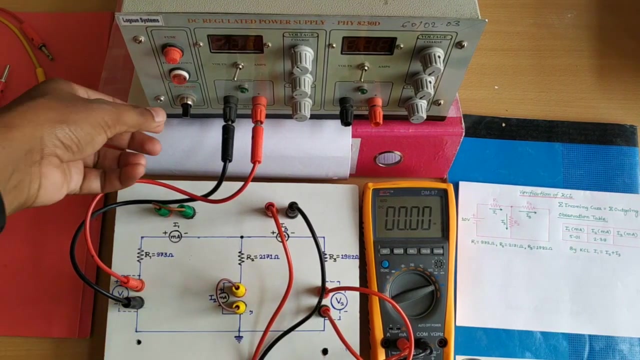 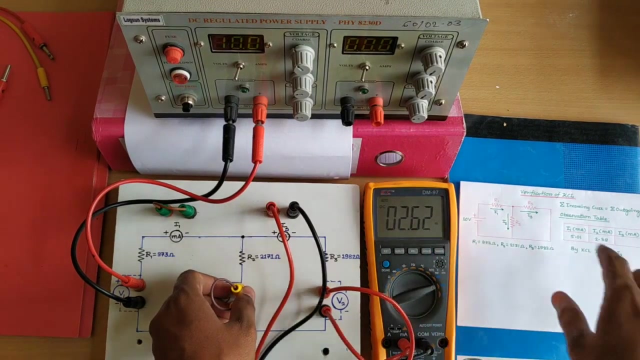 turn off the power supply and observe this reading pressing Shield. okay, and now i willamerate. i設 are now so the speechless on the power supply. and now, from now on, 2.62 milliampere. so this is nothing but your i3, so we will note down this value: 2.62 milliampere. 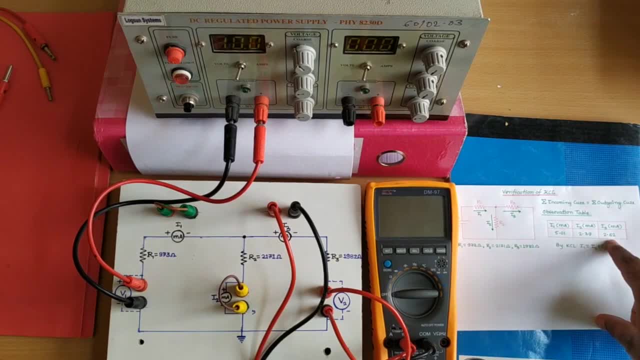 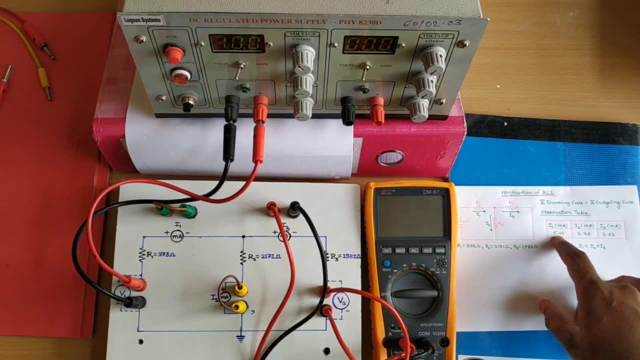 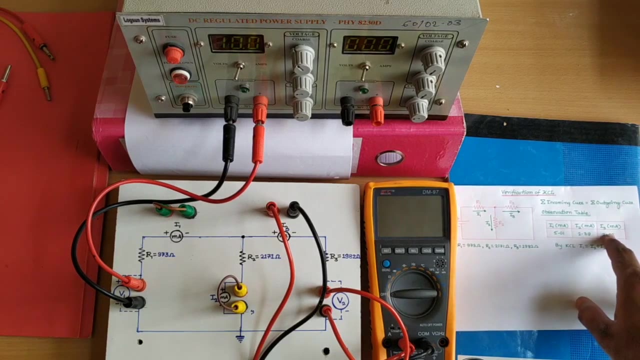 so here you can see that we have noted all three currents values. okay, now, according to the kcl, incoming current, what is incoming current i1- almost 5 milliampere- and what are outgoing currents- i2 and i3? so if we add these two currents, their addition should be equal to i1, because i1 is. 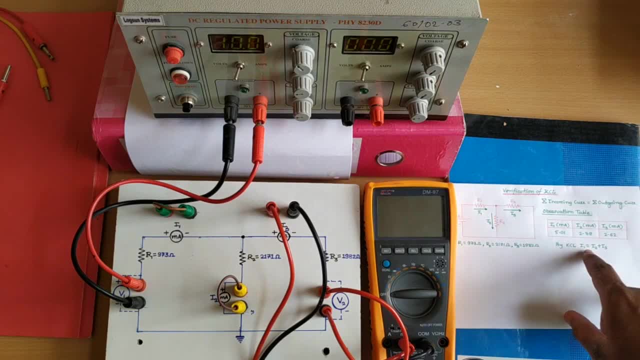 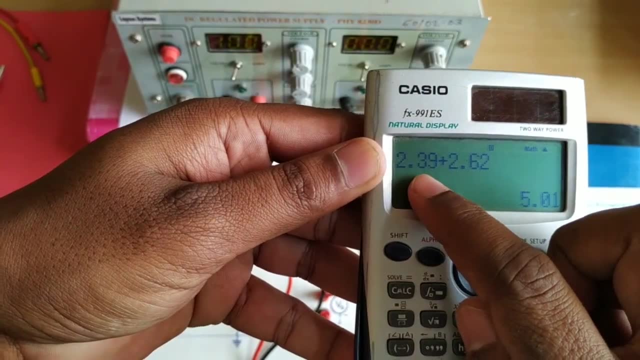 equal to i2 plus i3 according to kcl. so if this thing is verified, then we can say that our kirchhoff's current law is verified. so your i2 is 2.39, i3 is 2.62. if we add them what we are. 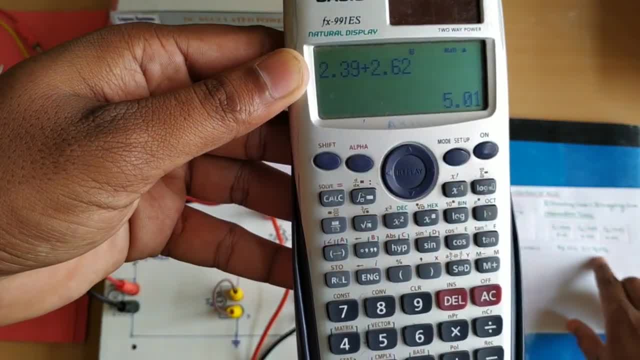 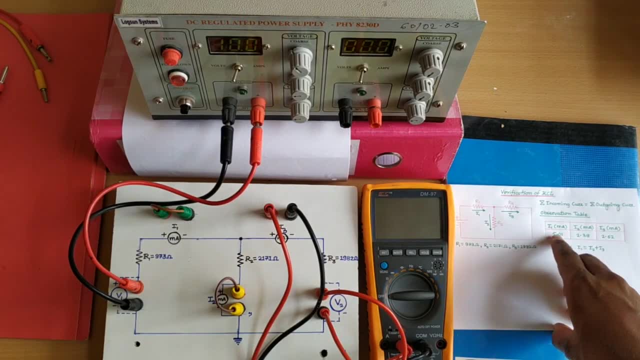 getting 5.01. okay, so what is your right hand side? so, if you look at this, what is your right hand side- 5.01- and what is your left hand side? i1 means again 5.01, so left side is equal to right side. 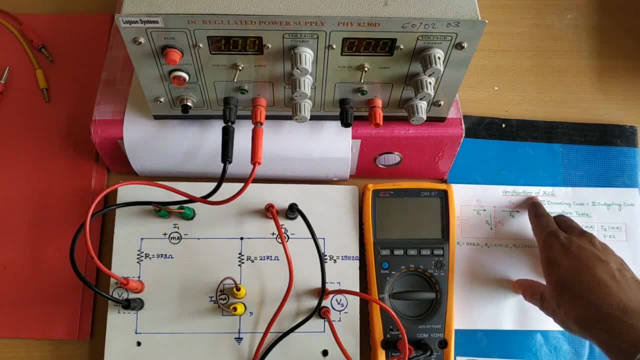 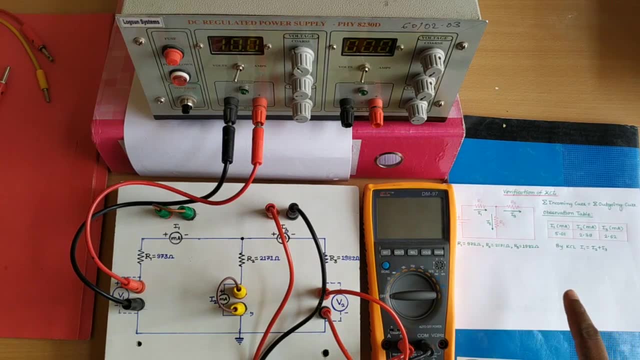 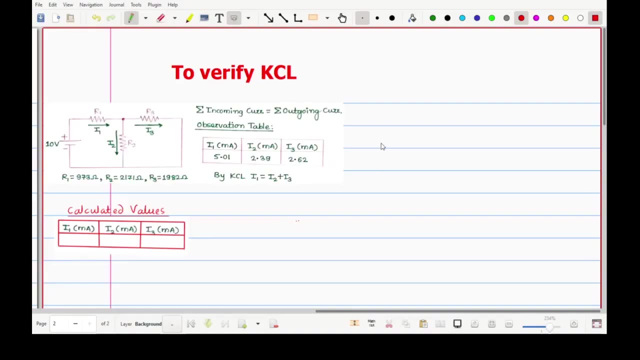 so this are same. hence our kirchhoff's current law is verified. practically okay means incoming current is equal to sum of outgoing currents. same law can be verified theoretically- okay. so for that purpose we will do the calculations in the next part. okay, so, friends, demonstration part is already. 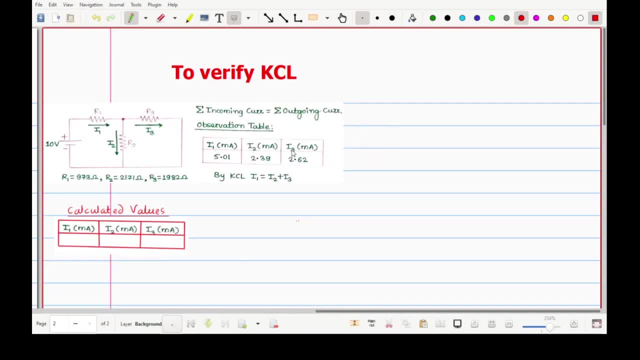 over now we will calculate the value of i1, i2 and i3. okay, theoretically, for that purpose we have to apply kcl at this node. okay, so what you can see over here, incoming current is i1. outgoing currents are i2 and i3. so, as for our statement, incoming current. 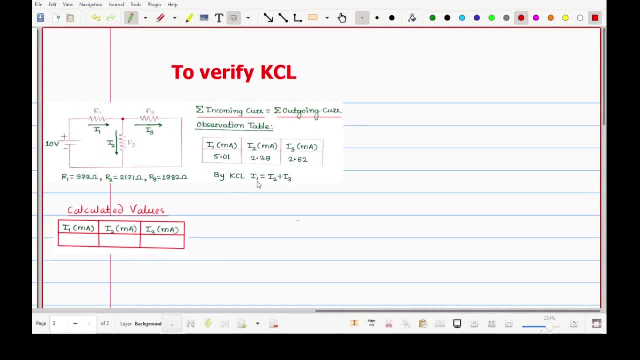 should be equal to outgoing current. okay, so if you apply this theorem, we are getting this equation. so if this equation is satisfied, we can say that our kcl is verified. okay, what you can observe over here, current i1 is coming, okay, and it is getting divided into two parts in between r2 and r3. so we 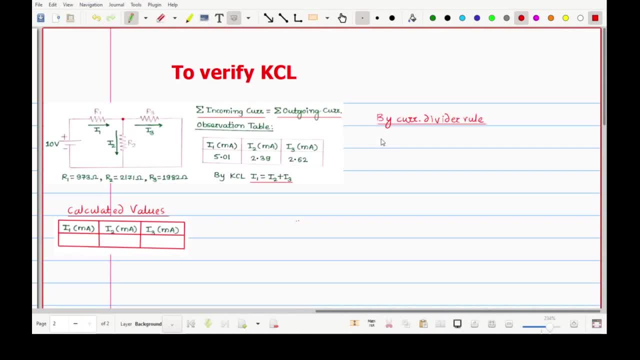 have to apply current divider rule over here. so by current divider rule we can calculate i2 as well as i3. so suppose we want to calculate i3 now. i3 is flowing through r3. so what is the opposite resistance r2. so i3 will be equal to what r2 upon r2 plus r3, okay, multiplied by total current. now. 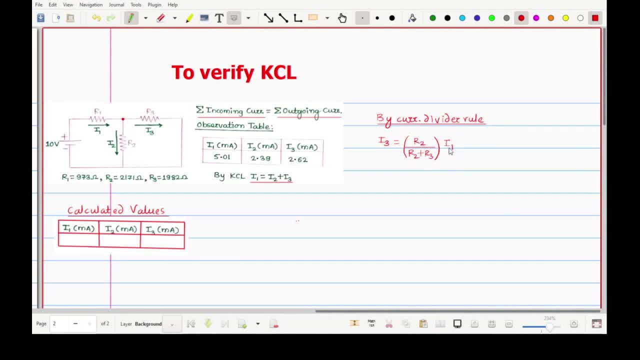 what is the total current incoming current i1. okay, so now we do not know the value of i1, so first of all we will calculate i1. so what is the i1 you are getting? it is equal to what total voltage upon total? what is the total voltage you are applying over here? 10 volt, okay, and what? 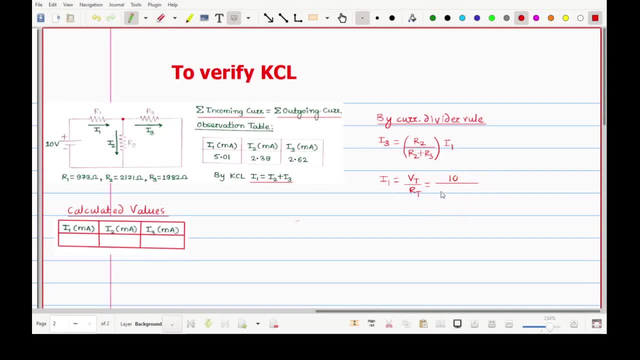 is the total resistance over here. so if you look at this, your R1 resistance is in series with parallel combination of R2 and R3. so this is the total resistance. we are getting R1 plus R2, parallel to R3. okay, now put these values and. 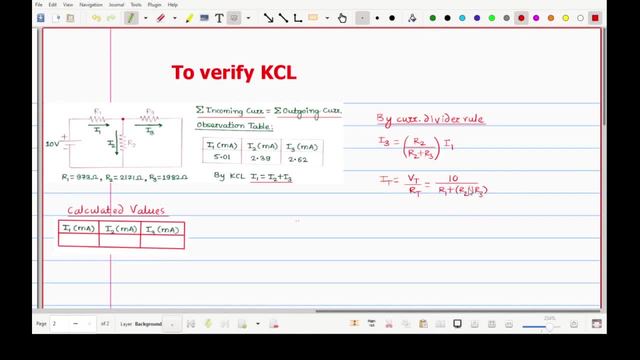 calculate this total current. okay, so this equation you are getting now calculate the value of IT. so here you will get 4.97 milliampere. okay, now put this value in above equation, you will get the value of I3. so when we put R2 and R3, 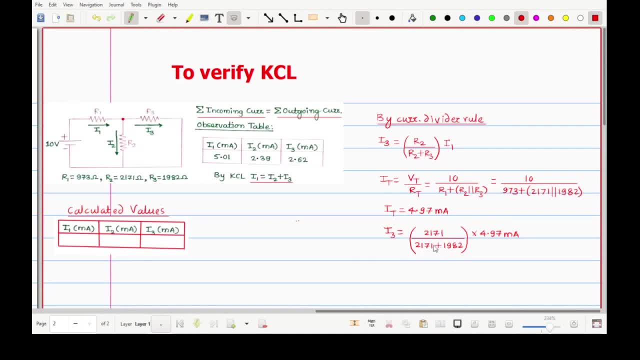 and total current. we are getting this equation. okay, so now calculate the value of I3, so you will get 2.60 milliampere. okay, so this is the value of I3. you are getting calculations. okay, so now down this value. so 2.60 milliampere we are getting. 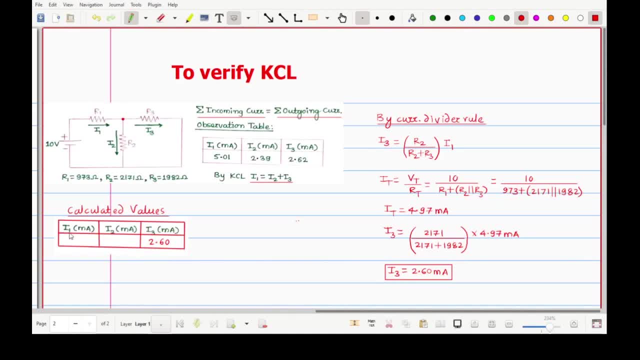 okay, now we know what is your total current. so your total current is nothing but what I1. okay, because here what we have written, the current which is coming from the supply, is nothing but what your total current. so IT and I1 are same. so I1 we have already calculated. so I1 is nothing but what. 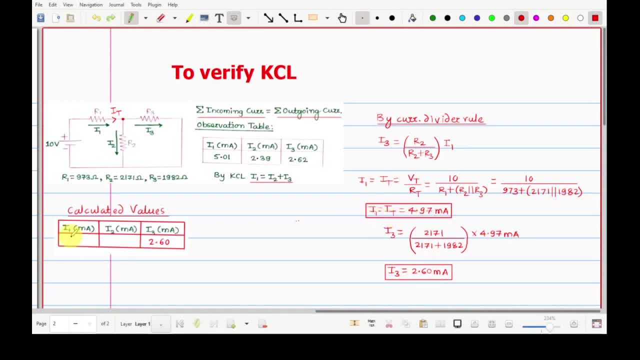 I2. so I2 is nothing but I1. so what? we are getting over here? 4.97 milliampere. you are getting okay, now what is remaining? I2, so okay. so what is the equation you are having? we are having this equation from KCL. okay, so I1. 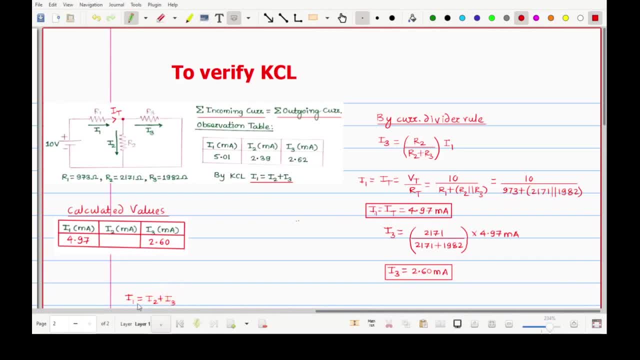 is your incoming current. it should be equal to outgoing current means, I2 plus I3. okay, so I1 and I3 are known to us, so this equation will give you what I2 so of both currents to calculate this. so, friends, if you calculate this, you will get i2 is equal.